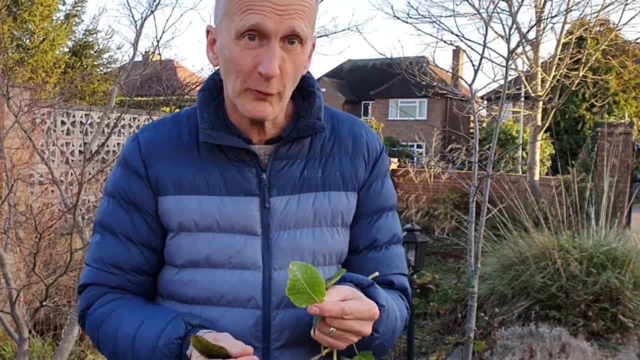 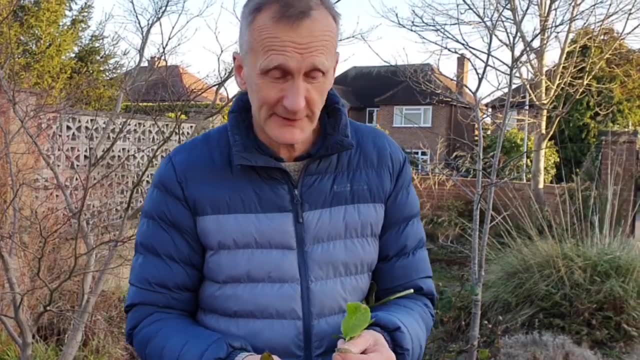 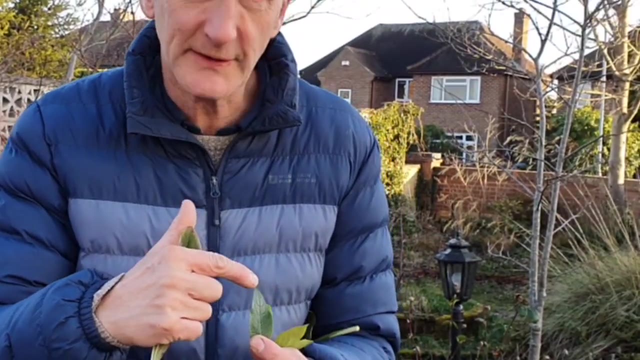 If there are really lots of them close together, we call that denticulate. Just think of your teeth denticulate. And for serrations, think of a serrated knife. And you can see here on the buddleia they're really finely serrate. 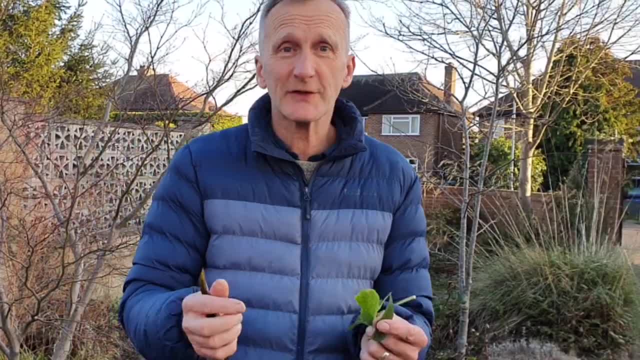 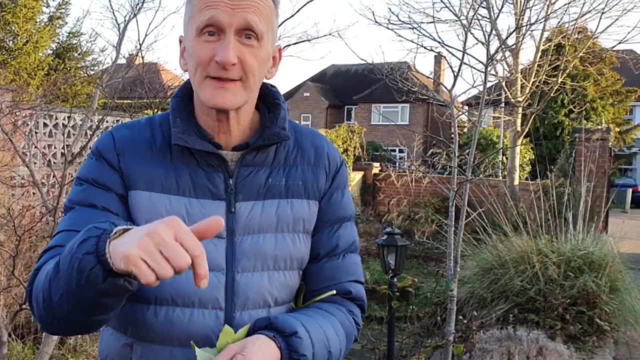 So that's called cerulate. So in this session we'll have a look at the leaf margins And, as in the previous weeks, there is a challenge below. So you click the button below And there'll be a Quizlet challenge where you can test yourself, see how you get on. 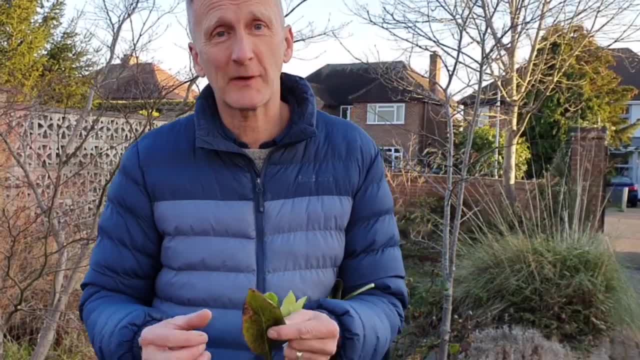 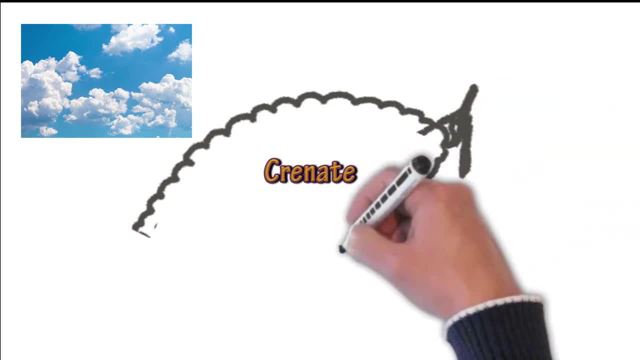 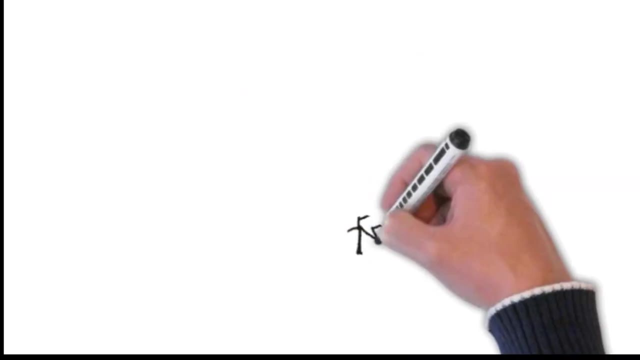 And then next week we'll look at another aspect of plant identification. So think of crenate as clouds just going round and round the outside, cloud-shaped, And that's a good way of remembering that particular term. And then we have another one which is just like the serrations. 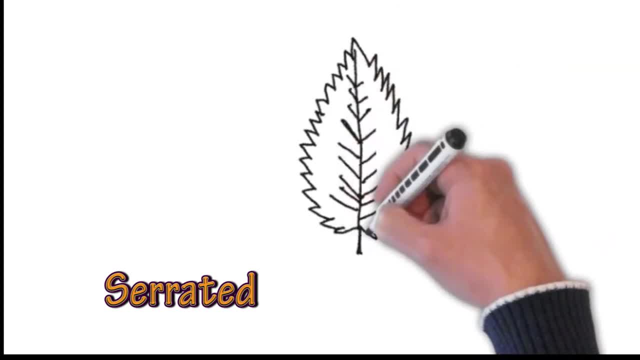 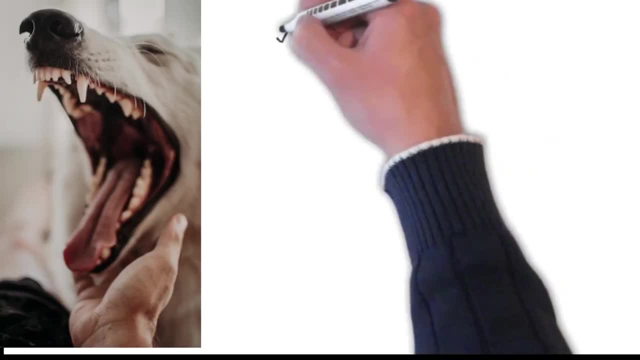 on the side of a knife if you look at the way the margin of that leaf is. So we call that serrated, like a serrated knife. And then the next one we're going to look at is what we call dentate. 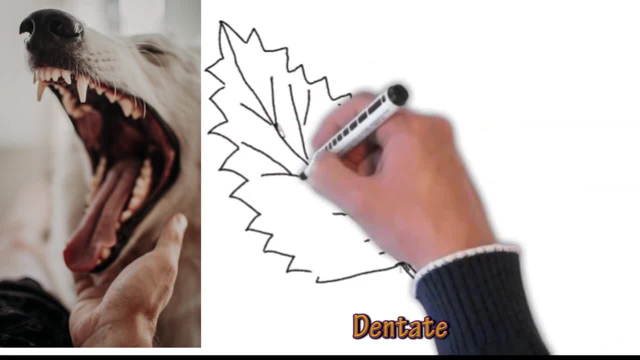 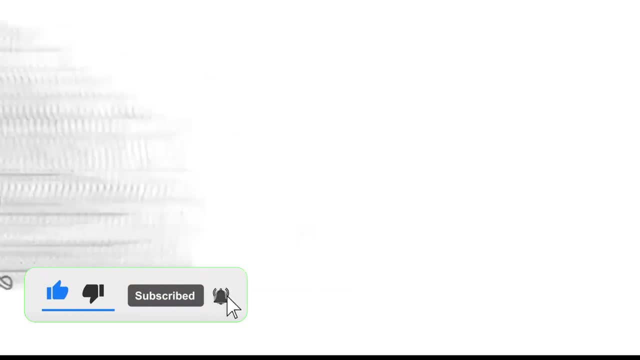 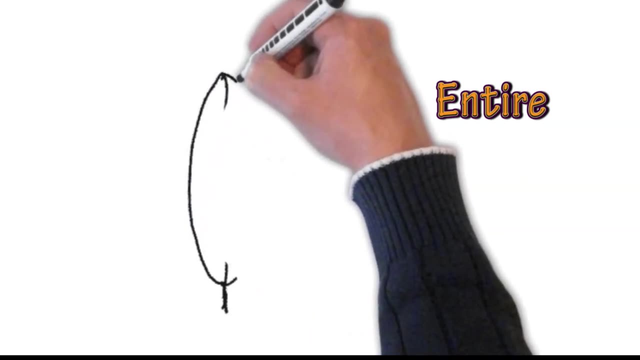 So think a dentist. or in this case, you can see the canine teeth on that dog to the left. So, dentist dentate looks like a dog's tooth on it. Now, if the side of the leaf is smooth, then we call that entire. 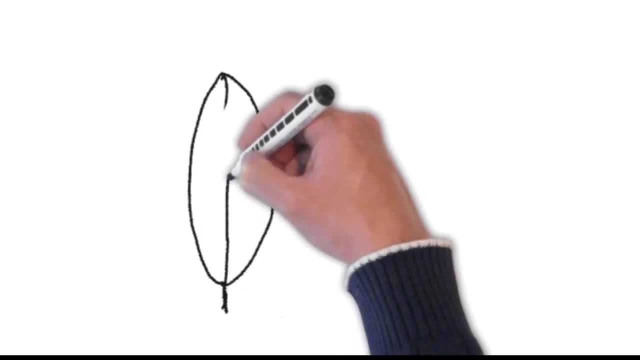 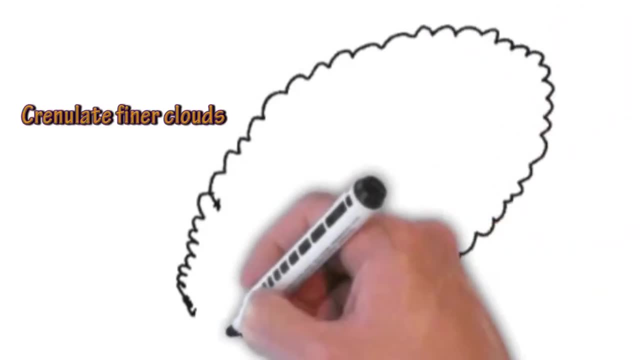 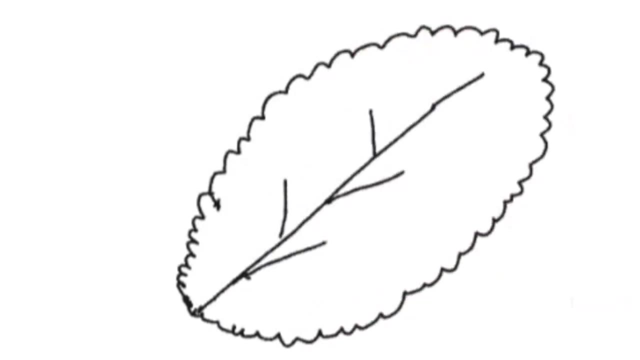 So it's smooth or entire, So that's a term that we often use. If the clouds are really fine and very close together, that's called crenulate, So really fine sort of little curvy bits around the outside, And if it's very finely serrated, 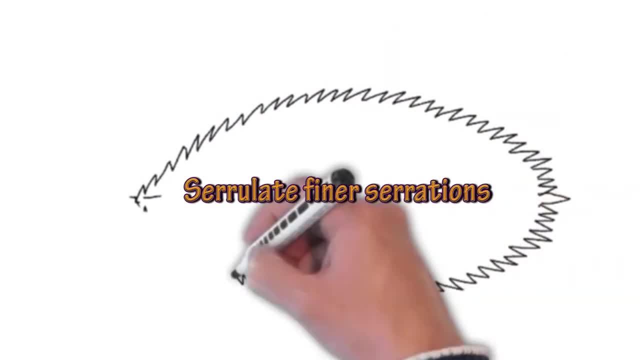 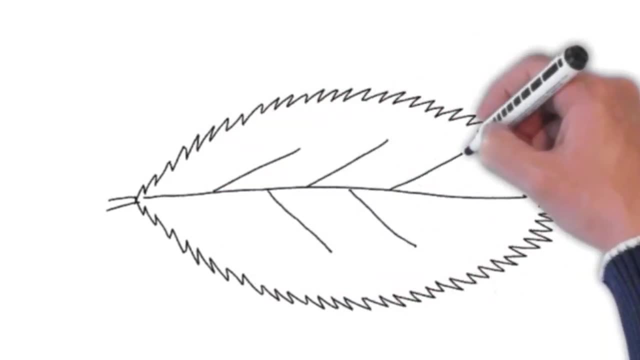 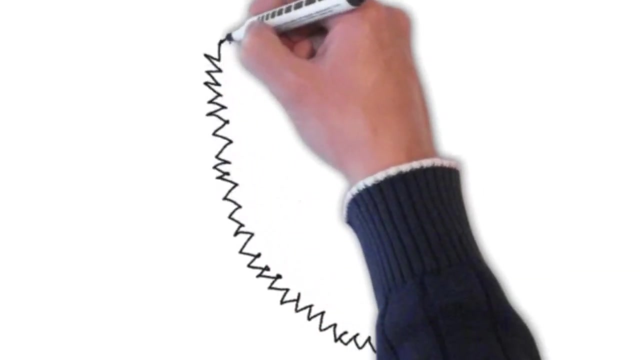 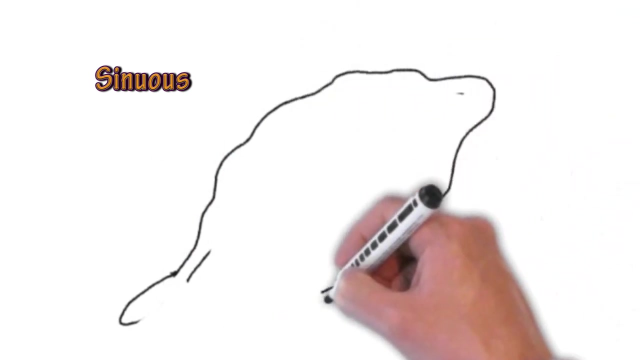 we call that cerulate, And if it was like the toothed one, then that's called denticulate. Another one that we would use is what's called sinuous, a slightly wavy margin around the outside If it goes up and down. they sometimes call that undulate. 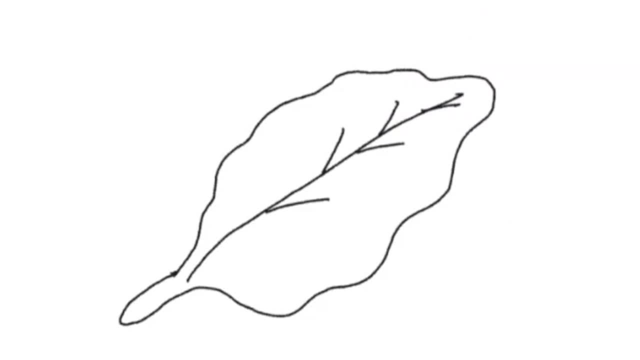 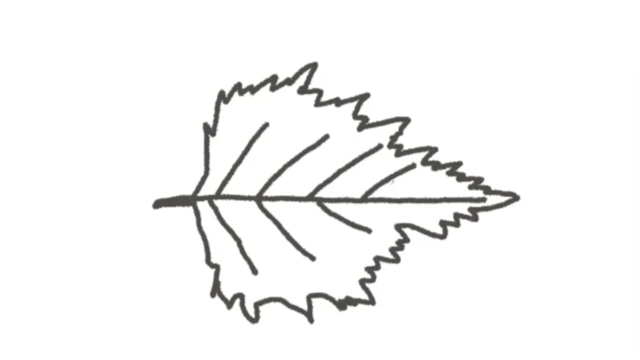 But if it's wavy around the edges it's sinuous. Another one that we see is where the serrations vary- small serration, big serration- And that's called a double serrated leaf, double serrated margin, if you like. 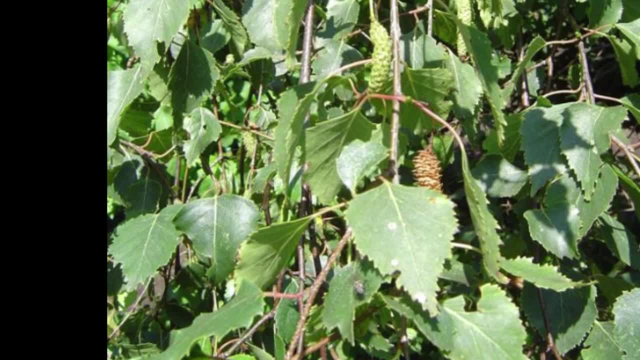 So the double serrate. we sometimes see that in Betula pendula. If you look on the right hand side of that leaf, in the middle it's got a small, then a slightly larger serration, And that's quite useful when you're identifying birches. 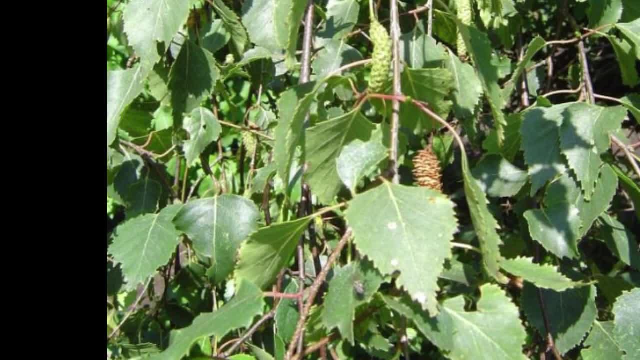 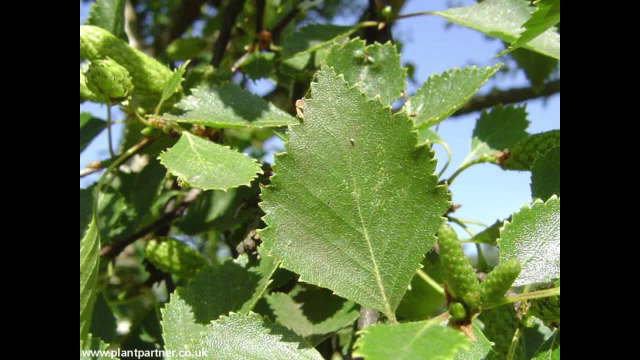 because Betula pendula is double serrate, Whereas if you look at Betula pubescent, the downy birch, then the leaf shape is different, in that it's slightly more diamond And the margin is pretty much dentate all the way around fairly evenly. 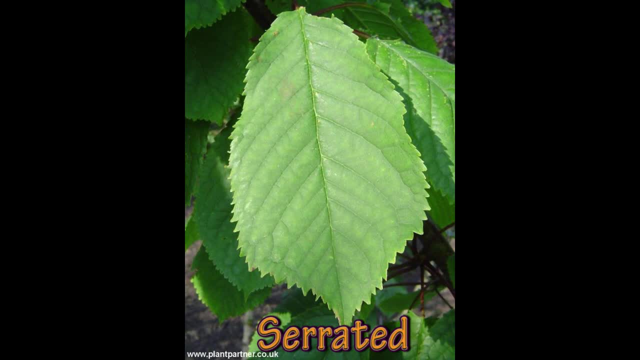 So the cherry tree Prunus. this has a serrated margin, So that's fairly common on a lot of rosaceous plants like the Prunus or Malus and that kind of thing. Onto the Oleria macrodonta, the daisy bush. 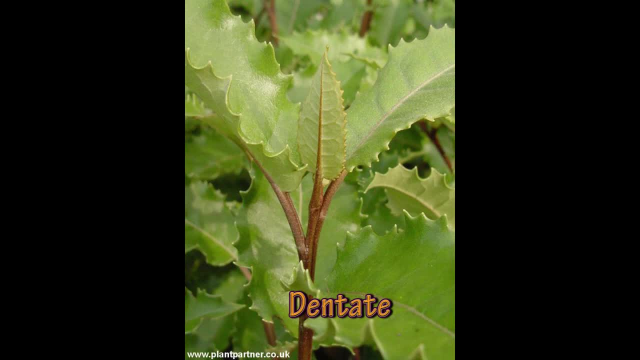 that has dentate type leaf. Look, they're quite toothed. So macrodonta large teeth is the botanical name for that one. On the grisolinia you can see that the leaf is very smooth, So that's what we call entire. 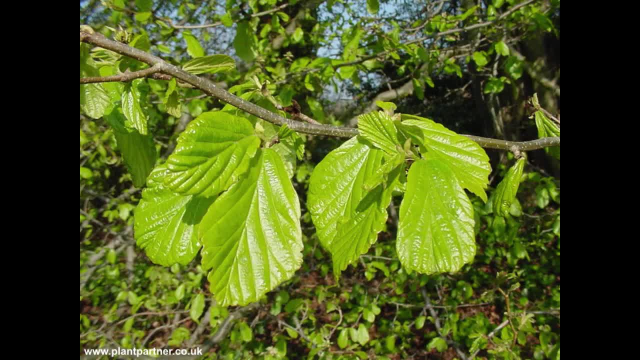 So it's smooth all the way around. Prusia, persica, the Persian ironwood. as you can see if you look closely, that's got a crenate margin, a cloudy shaped one. So onto the Deutzia. you can see here. 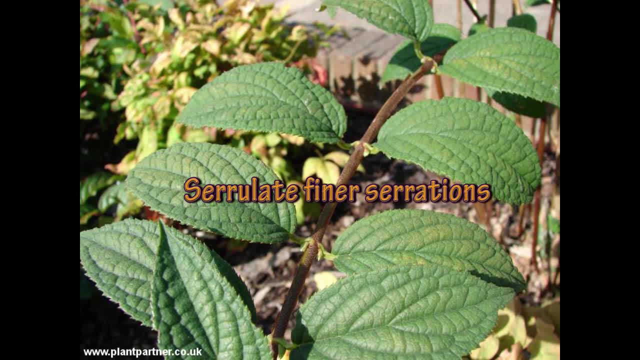 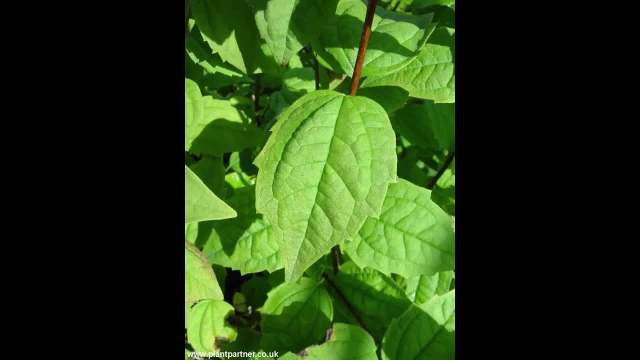 it's got a very finely serrated leaf, So we'd call that cerulate leaf. It's a little bit finer than the larger serrated one Onto the Philadelphus And you can see that the bottom of the leaf is entire. 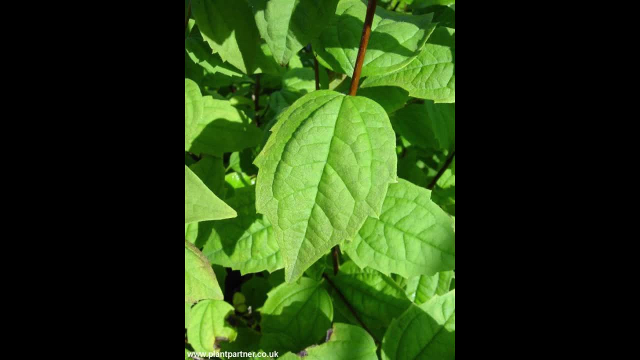 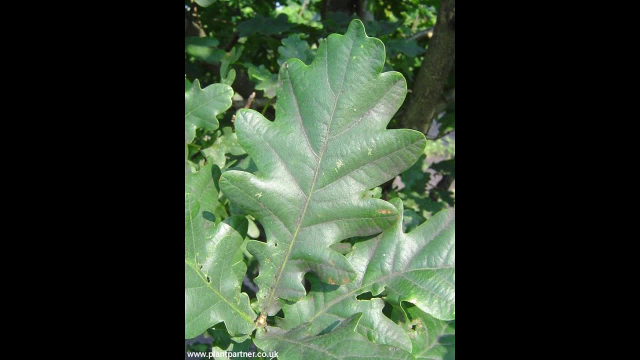 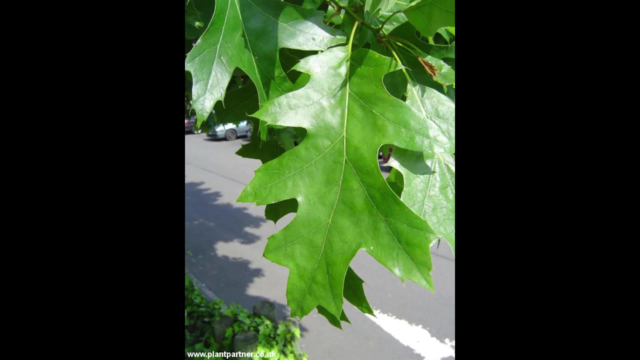 It's quite smooth. but then it goes into a kind of sort of serrated for the top two thirds of the leaf And then we have lobed on the oak. That's the actual shape, not the leaf margin With the. so that was Quercis ruber.